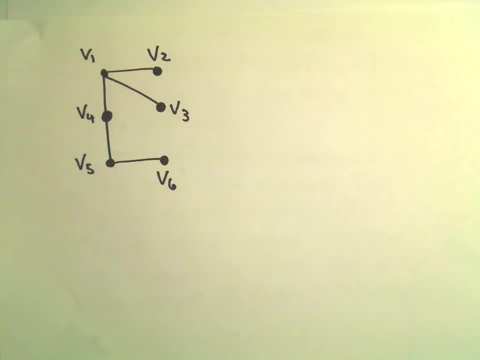 That's all. a graph is Okay. So we talk about graph theory. We're not talking about Y equals X, squared, Just points and lines connecting them. So we would say: the vertex set V for this graph- maybe we'll call it G- are just V1, V2, V3, V4,, V5, and V6.. 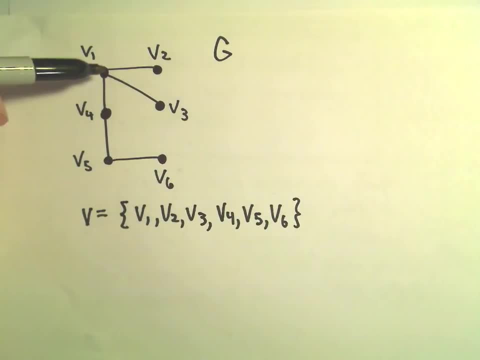 And you can think really, you know, maybe these are just six people at a party and V1 knows V2, V3, V4. You can see that V5 only knows person V4 and V6. Maybe that's what an edge represents, is if they know each other okay. 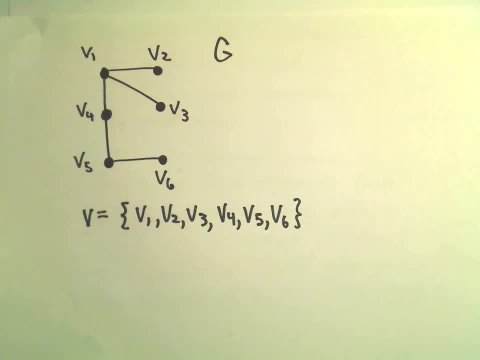 You know, and you can make the edges represent whatever you want to. So maybe we'll just think about the edges as meaning there's a connection between them and they know each other. So the edge set that's just going to be all two element subsets. 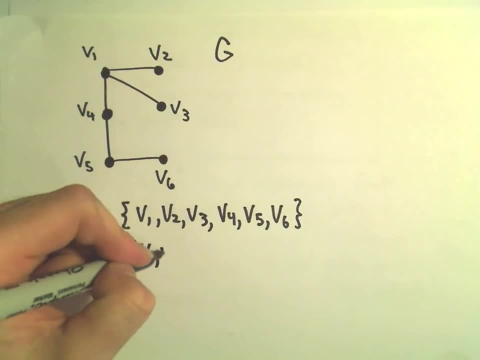 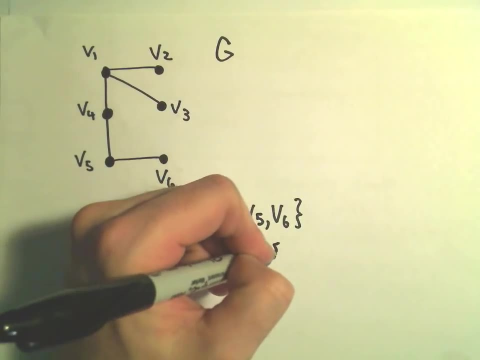 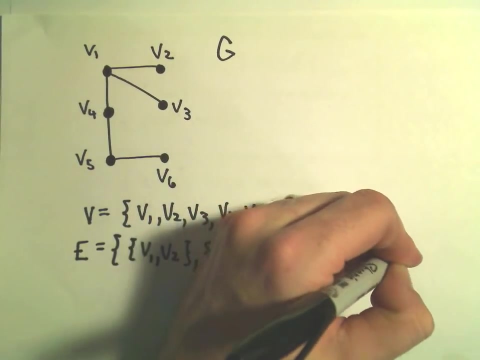 And basically we just list All the vertices that have an edge between them. So V1 and V2.. V1 and V3.. V1 and V4.. Let's see, V4 is connected to V5. And then vertex V5 is connected to V6. 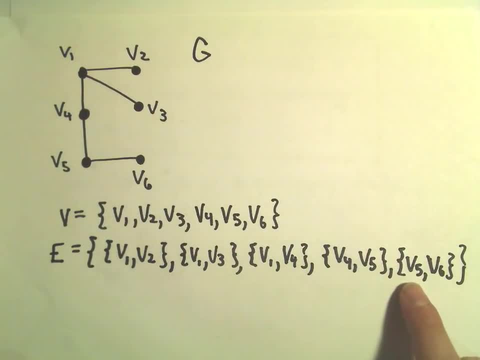 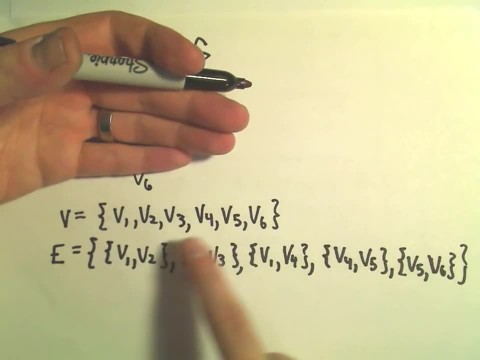 And I think that's everything we need. You know we don't need to list: V6 is connected to V5, for example. It's just redundant already. So If I had you know again, basically just this set and this set E. 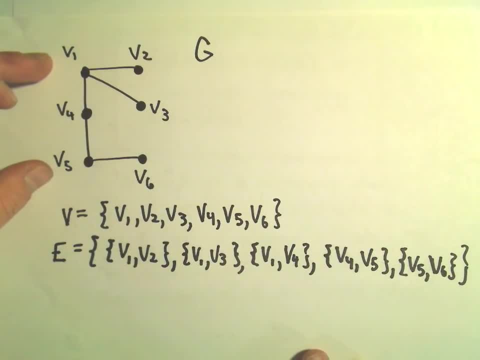 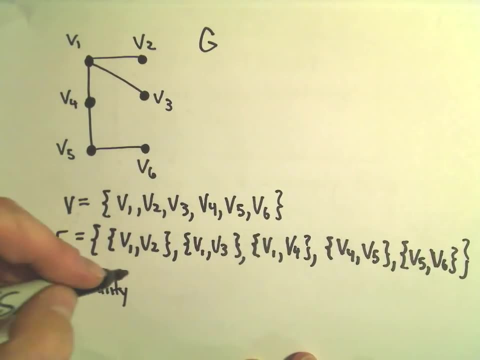 Again, it's just basically telling me all the information in this original graph. So I still know that. A couple things: The cardinality: The cardinality of a graph just represents the number of vertices. The notation I've seen is they'll put an absolute value. 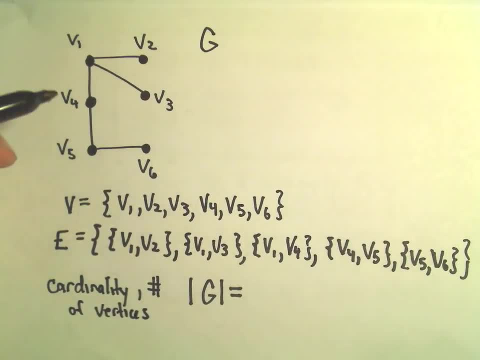 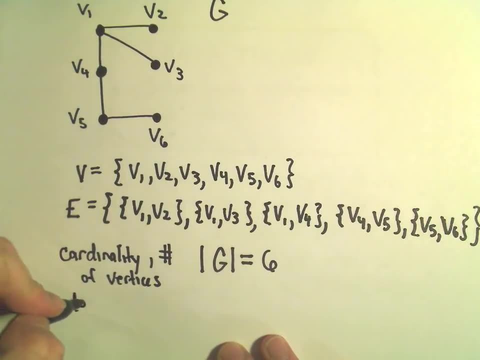 So the absolute value of G, The cardinality of G, is just the number of vertices, Which in this case is In this case, is 6.. Let's see: Another thing that we often talk about is the degree of a vertex. 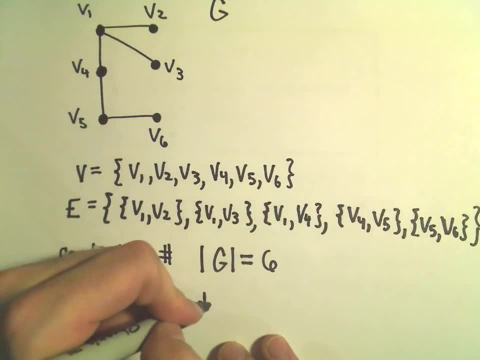 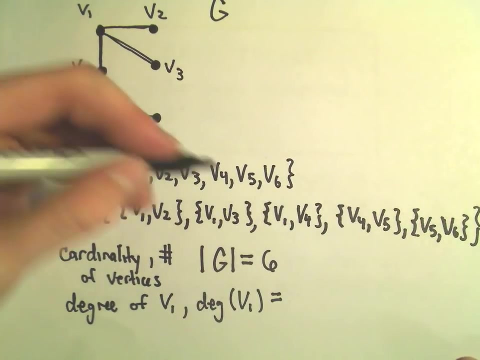 So, for example, the degree of vertex V1. Which they'll abbreviate little D, E, G, V1. All that tells you is the number of edges coming out from vertex V1. So there's 1,, 2, 3 edges leaving V1.. 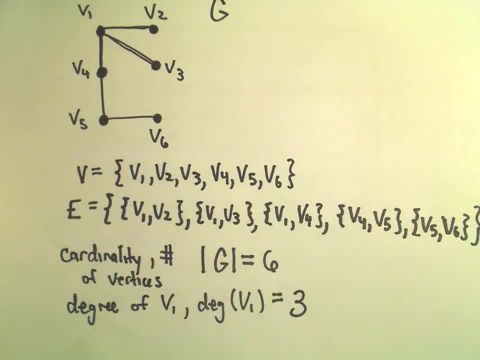 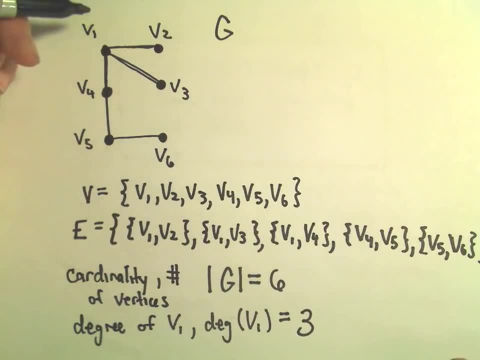 So we would say the degree of vertex V1 is 3.. Again, so vertex V1 knows 3 other people is all that says. Another kind of convention for a typical graph. We don't let a vertex have a loop back to itself. 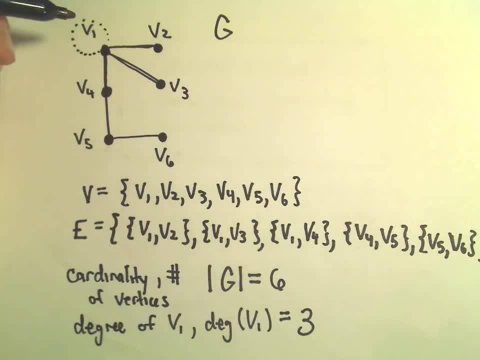 Okay, I mean definitely. that certainly happens in a lot of applications. But when we allow graphs to have loops back to themselves, Typically people will call those multigraphs. So multigraphs have loops. Regular graphs don't have loops. 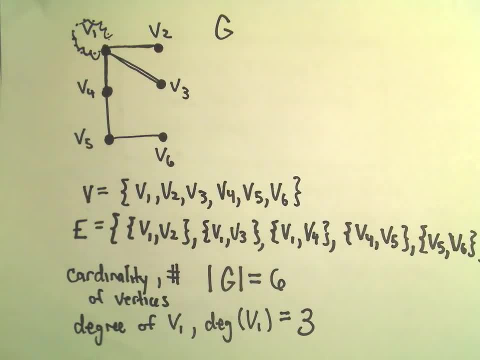 So pretend that loop's not there And we just got the original matrix, that we The original graph. we started with A couple other things too. The way that you draw the graph is irrelevant. So here's V1.. Here's V2.. 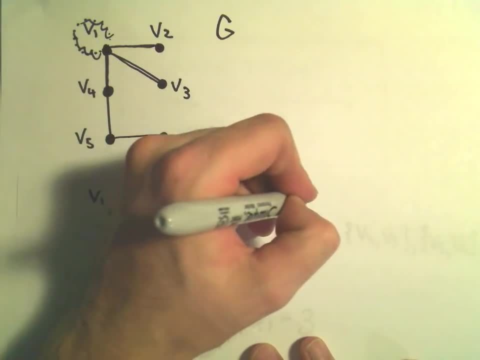 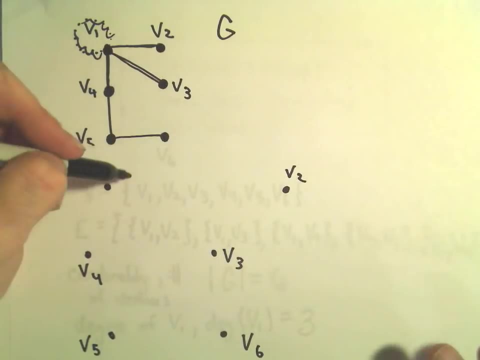 Here's V3.. Here's V4.. We'll stick V5 down there, I don't want to make it too crazy. V6. You know they don't have to be straight lines, They can be whatever they want, So okay. 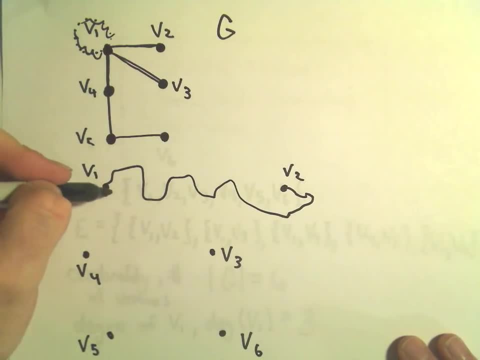 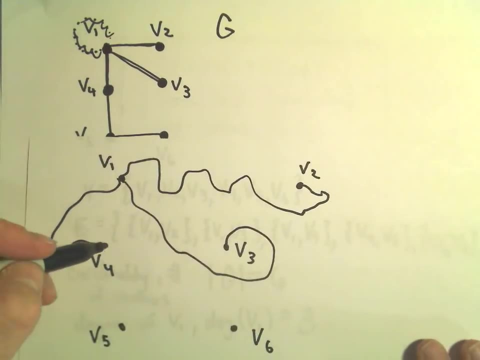 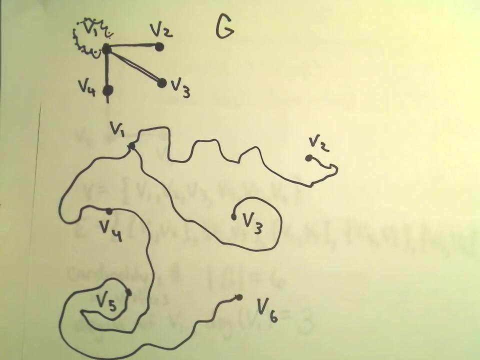 So V1 is still connected to V2.. V1 should still be connected to V3.. V1 is still connected to V4.. We'll have V4 still connected to V5.. And hey, V5 is still connected to vertex V6. 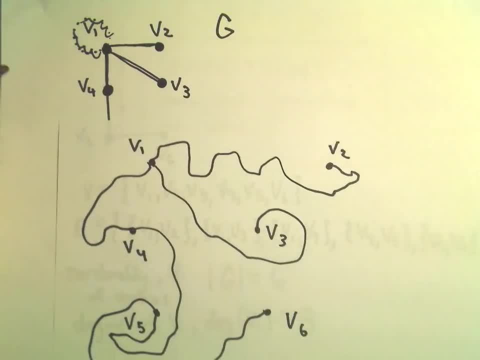 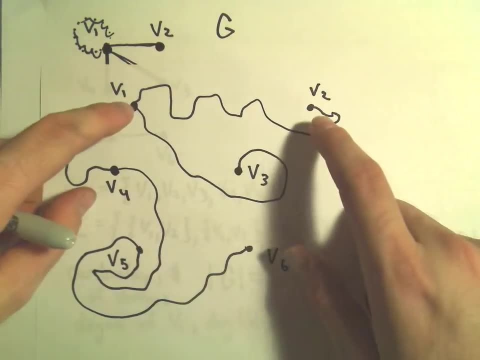 So all the original connections are still preserved And there's sort of no new connections in there that weren't there before. So when you have a graph where basically all the original information is preserved- The original connections, There's no new connections. 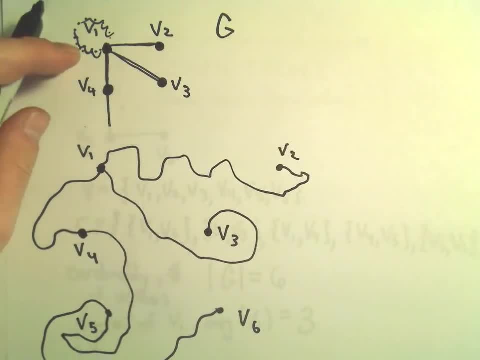 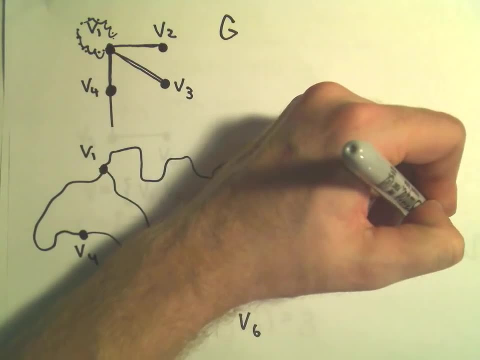 There's nothing missing, And again, this is a very kind of loose definition, But we would say that the original graph and this new graph are isomorphic, And all that means is, from a graph theory point of view, they're one and the same. 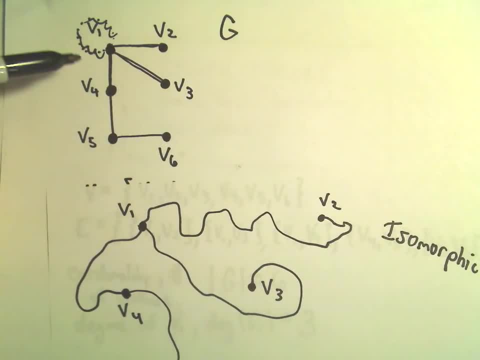 They're exactly the same graph. Okay, So typically, you know, we'll try to draw them, as a you know, in the least confusing manners possible. Okay, So, typically, you know, we'll try to draw them, as a you know, in the least confusing manners possible. 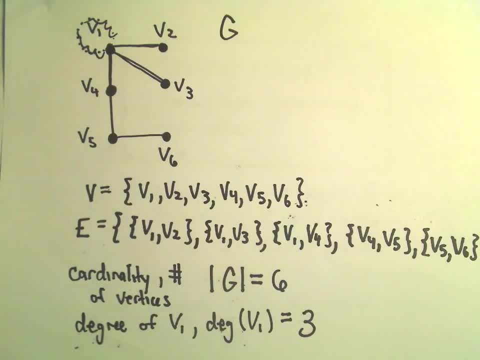 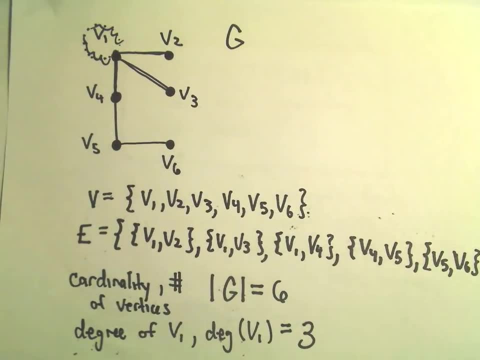 But definitely an important idea. The way that you draw the graph in general doesn't matter. Let's talk about a couple other ideas. just a way to describe a graph. One way is with what's called an adjacency list, And I don't know how useful these are. 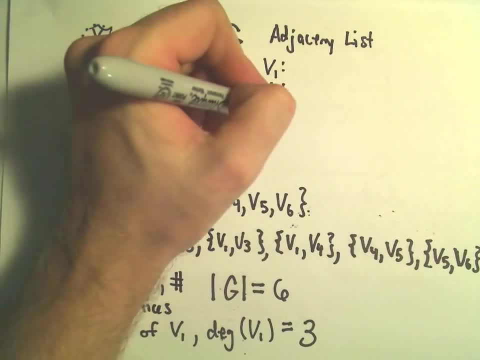 I never really saw them much. But again, I didn't take a tremendous amount of graph theory. So that doesn't mean that they don't get used all the time. So that doesn't mean that they don't get used all the time. 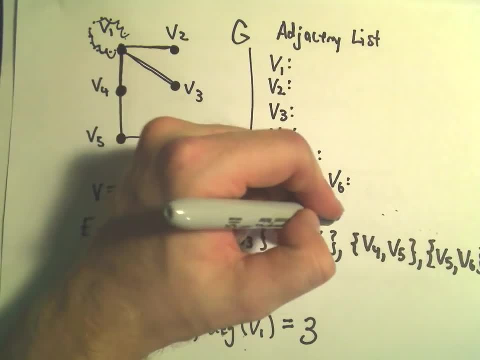 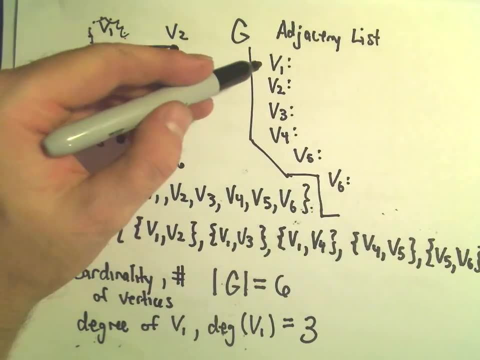 And I just haven't ran into it, But all an adjacency list is exactly what you think. So all we do is just list vertices that are adjacent. So for V1, it's adjacent to V1.. Excuse me, V1 is adjacent to V2,, V3, and V4., 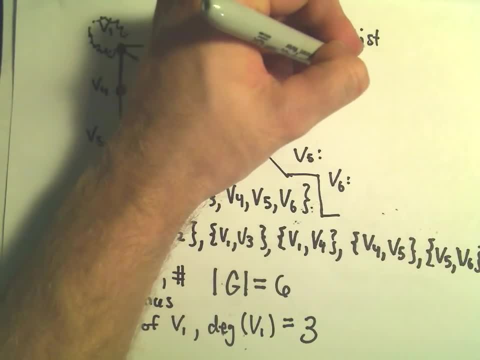 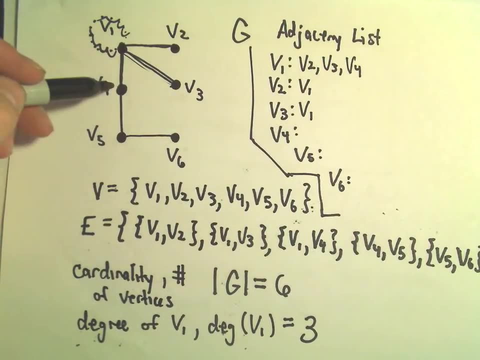 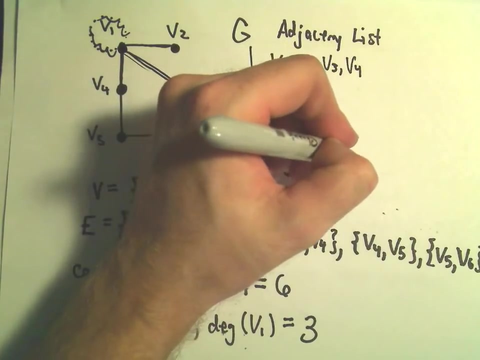 So we'll list those: V2, V3, V4.. Vertex: V2 is only adjacent to V1.. V3 is only connected to V1.. V4 is connected to V1 and V5.. V5 is connected to V4 and V6.. 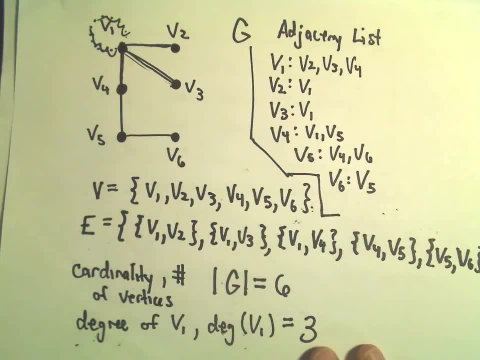 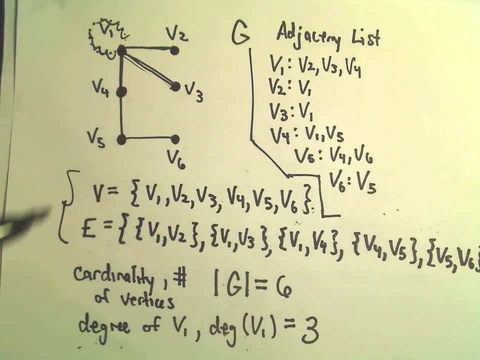 And V6 is connected to V5.. And again, it's just another way of summarizing. So this adjacency list, this set V and this set E and this graph again, are telling me all the exact same information. 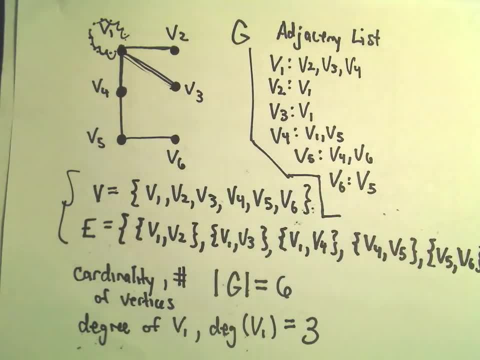 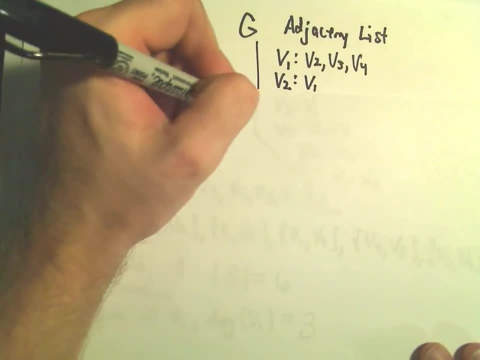 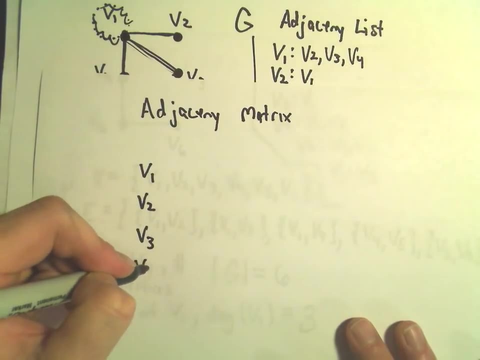 Another way that I know gets used all the time is, instead of doing an adjacency list, I'm going to make what's called an adjacency matrix. Okay, So I'm going to imagine V1,, V2, V3.. Typically, people won't even write these. 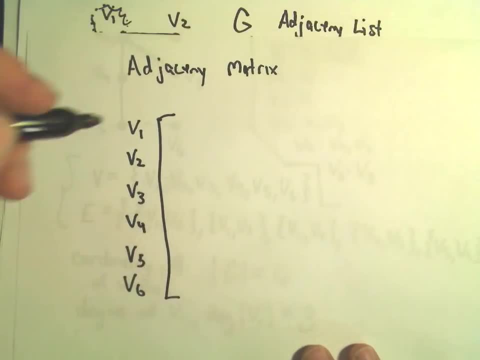 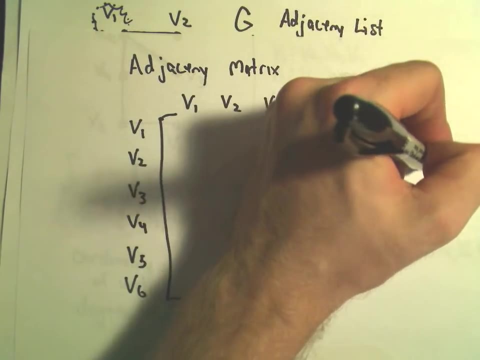 but you know, this is what makes sense to me. So a lot of times I used to always stick them in there: V1,, V2,, V3,, V4,, V5, and V6.. All we do is if there's a loop. 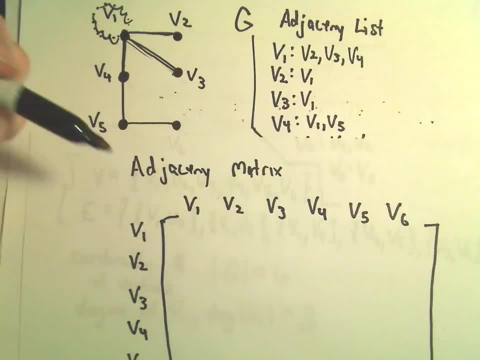 if there's a connection from a vertex to another vertex, we'll put a 1.. And if there's not, we'll put a 0.. So since there's not a loop from V1 to V1, we'll put a 0 there. 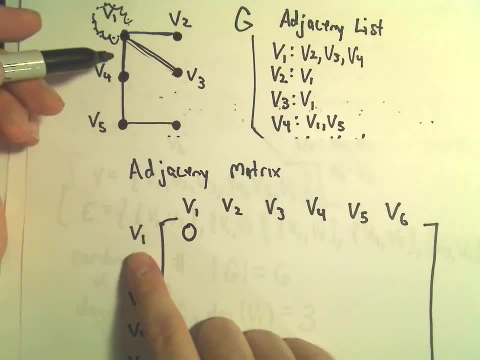 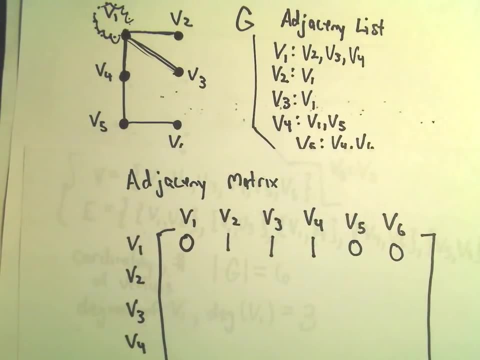 But V1 is connected to V2, V3, and V4. So V1 is connected to V2, V3, and V4. But it's not connected to V5 or V6. There's not an edge present. 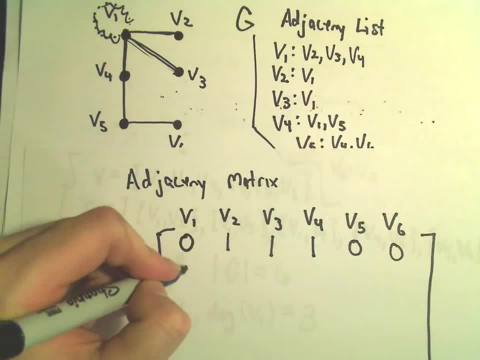 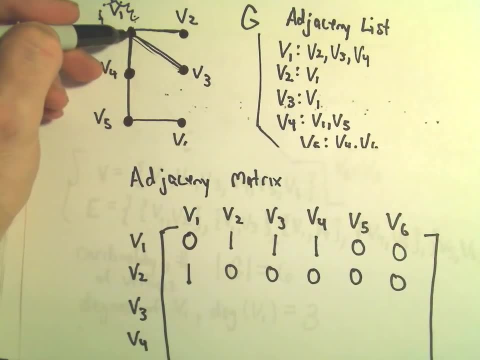 Likewise, V2 is only connected to V1, so we'll put a 1 there, And then we'll put 0s everywhere else. Let's see, V3 is also only connected to V1, so we'll put a 1 there. 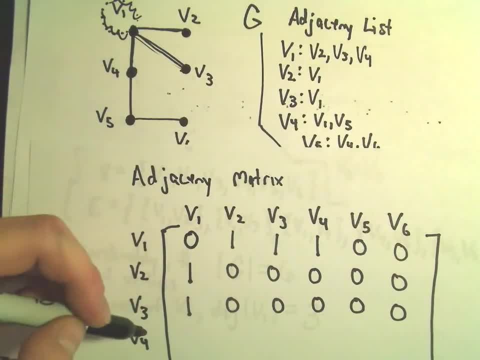 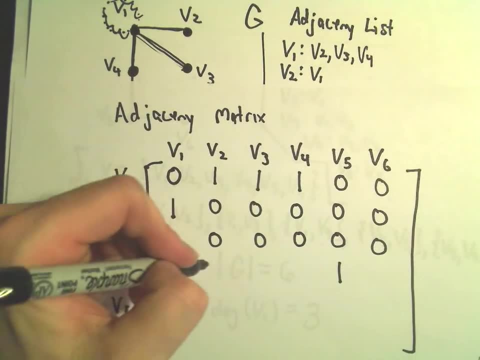 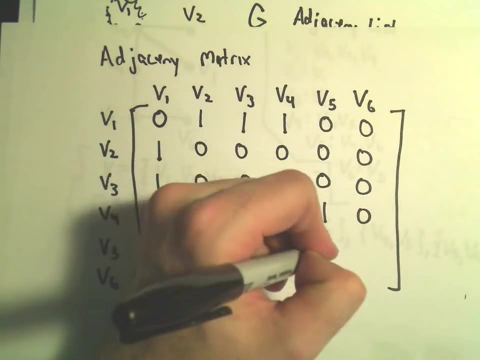 and 0s everywhere else. V4 is connected to V1 and also to V5, so we'll put 1s there, 0s everywhere else. V5 is connected to V4 and V6, so we'll put 1s there, 0s everywhere else. 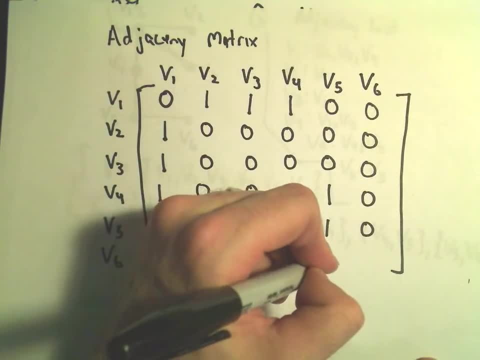 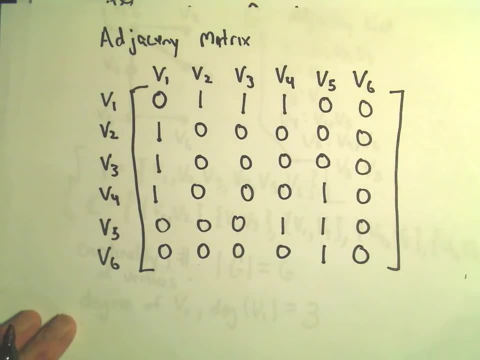 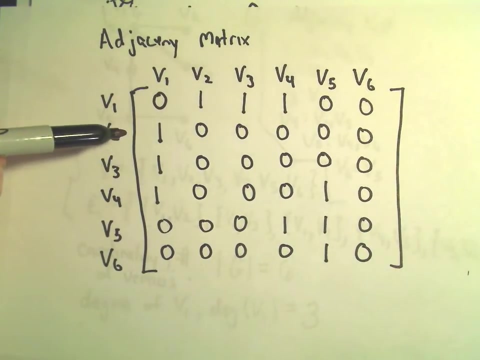 Lastly, V6 is only connected to V5, so we'll put a 1 there and 0s everywhere else. So this is nice because you can do math with matrices. So definitely there's a lot of study done with matrix representations of graphs. 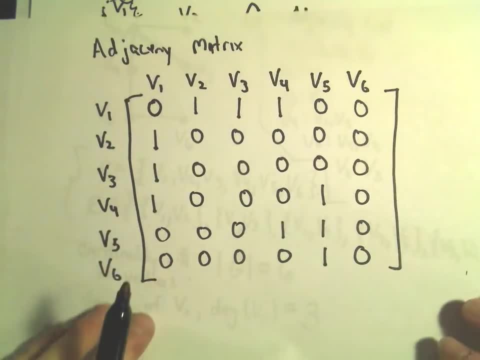 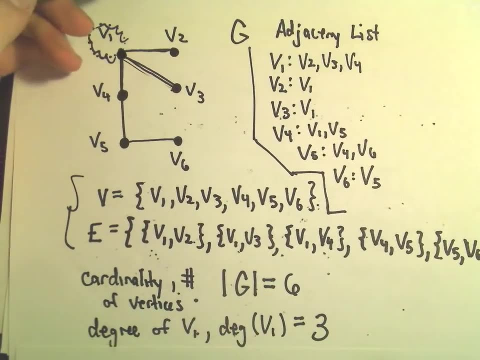 You can do stuff with that. Two last things, just maybe two last ideas. Notice for any vertex here, if you You know so imagine maybe these are islands now and there's a little bridge connecting the islands, Notice in this graph. 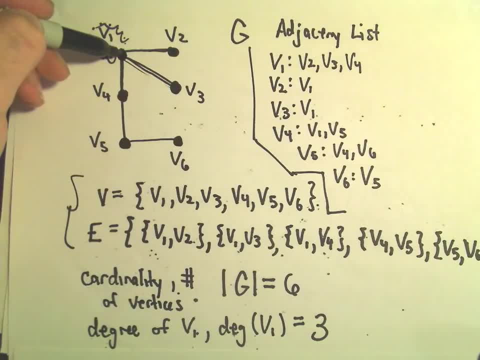 if you ever were to leave an island. suppose I was at island V1 and I went to island V4. The only way I can get back to island V1 is to sort of backtrack. You know, I could go all the way to V5 and V6,. 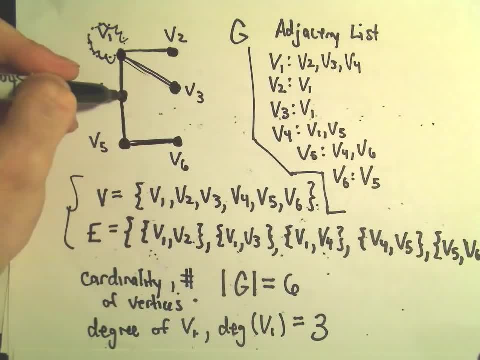 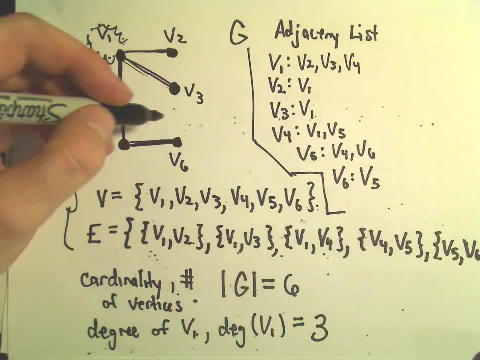 but eventually to get back, I have to take, you know, the bridges back, So there's no loops or what are called circuits. If there are no loops or circuits, we say that this is an example of a what's called a tree. 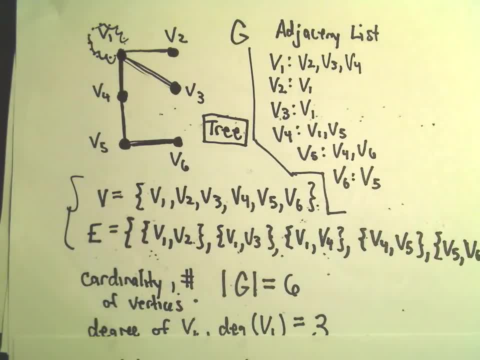 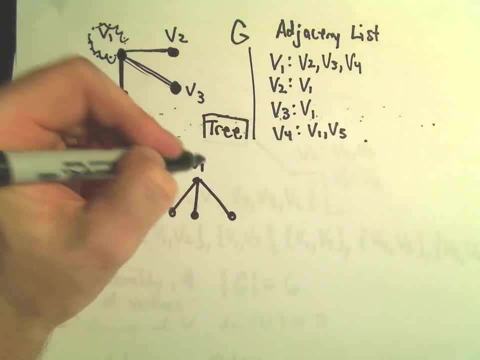 And the idea with trees is you can always sort of rewrite them, And the reason why we call them trees is we sort of can rewrite them, You know. so here's V1.. It's connected to V2, V3, V4.. 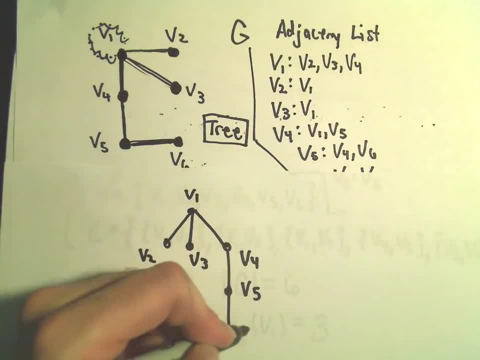 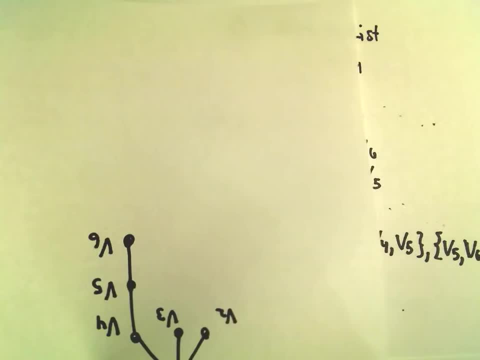 V4 is connected to V5, and V5 is connected to V6. So again, these would be isomorphic graphs, but now it kind of, if you flip it over and maybe it had some more branches, the idea is it starts to look like a tree. 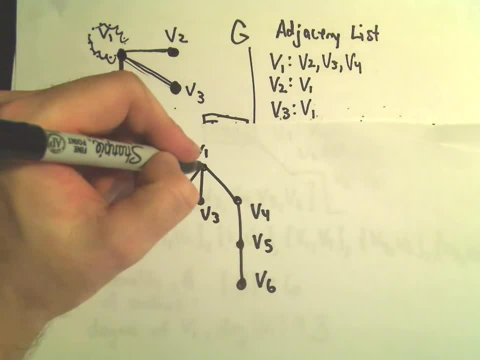 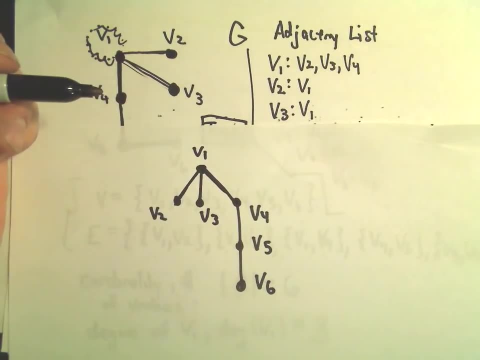 Trees get used all the time, For example. you know, imagine a chess algorithm. You know it's the first move. You know, maybe you've got one, two, three reasonable moves at your disposable. at your disposal, Not disposable. 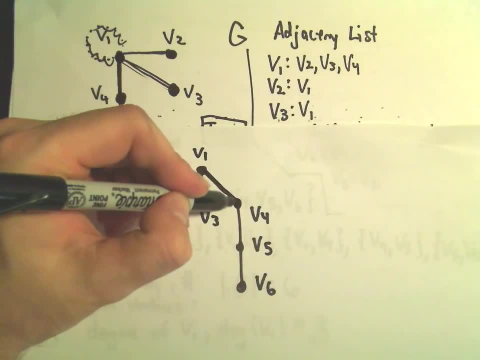 At your disposal. You know, and then maybe you know, once you consider this move, maybe there's only one logical move from that, and then from that there's only one logical move. So trees can help sort of represent, sort of searches. 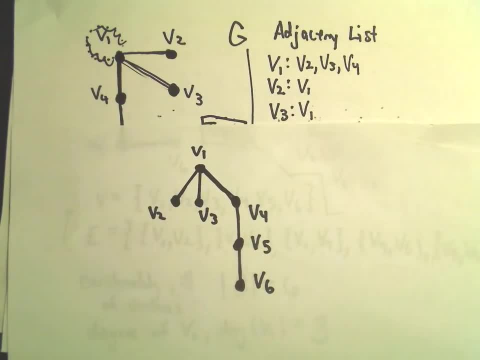 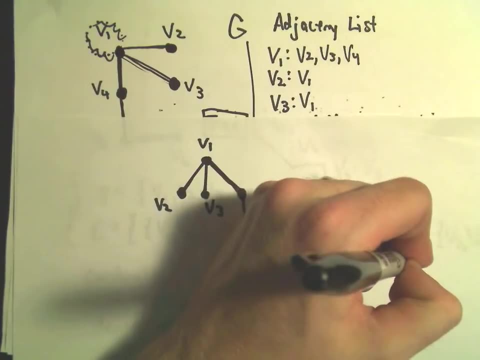 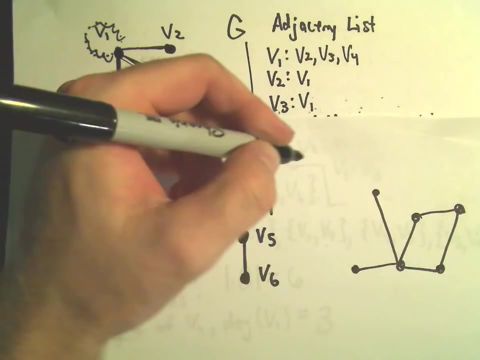 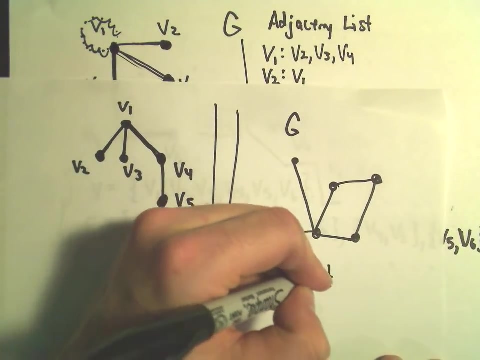 you know a computer search, So definitely one place. I know for sure that they get studied Again. if a graph, So maybe this is a whole separate little graph over here. This graph, we would say, has a circuit And the idea is a circuit. 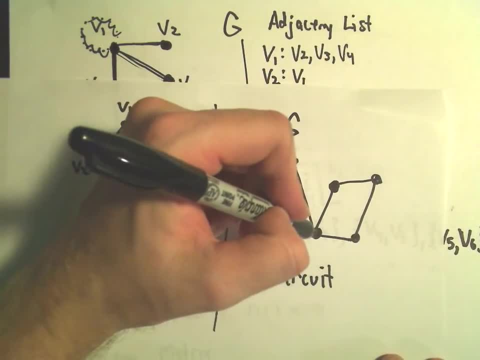 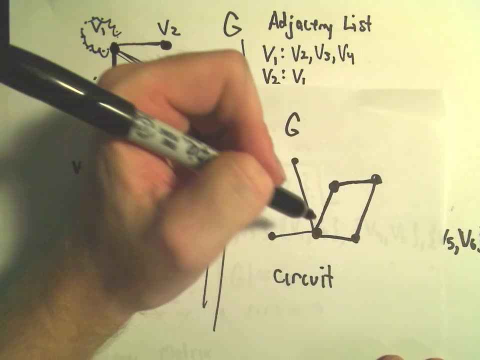 you know, for example, if I'm at this vertex, I can leave that vertex and still manage to get back to it without really ever backtracking through an edge or a vertice. I don't have to visit the same place twice, is all it says. okay. 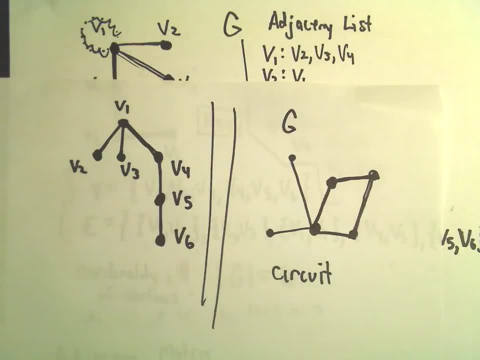 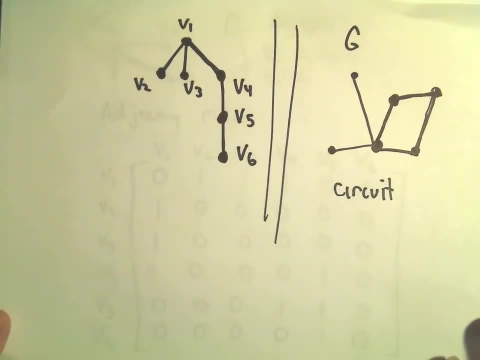 So this would be an example of a graph that does have a circuit. So graph theory, I think, is really interesting. You know there's tons of open problems If you're a budding math professor, if you're a math person out there. 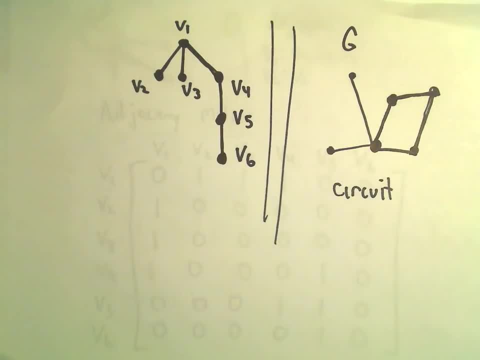 and want some challenging problems. there's definitely tons of open graph theory problems that are very simple to understand. You know, definitely you've got to learn some of the techniques to be able to attack things, but a lot of it is very sort of intuitive. 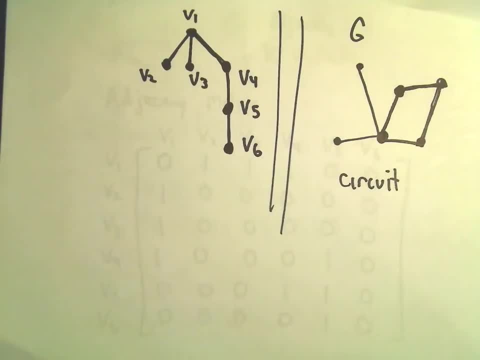 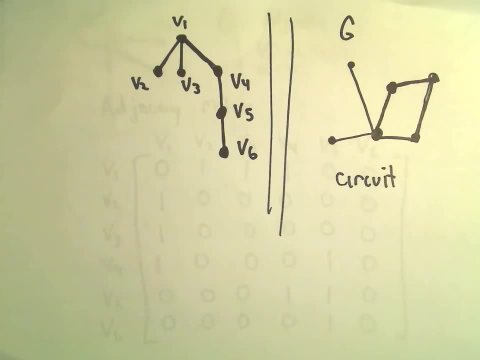 and I think open, you know sort of It's very user-friendly, is what I'm trying to say. There's still some reasonable open problems out there for people to tackle for sure. So if you are interested in kind of getting your hands wet, 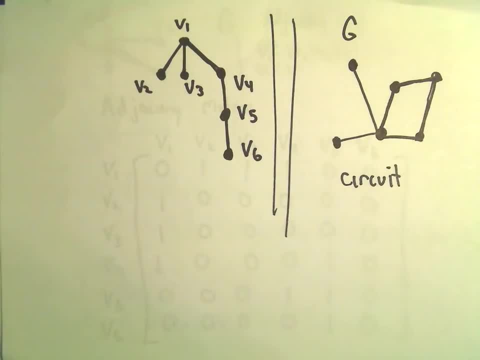 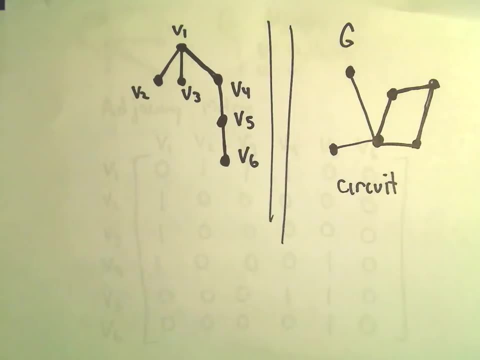 and doing some harder problems. I say graph theory is a great place to start. Maybe I can even post some open questions. So all right, I hope this little introduction makes some sense. Again, nothing too heavy. I definitely plan on doing some more. 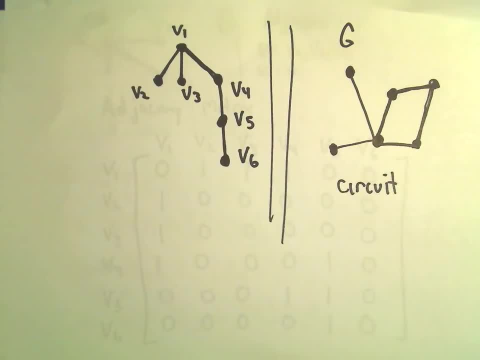 you know detailed stuff. But again, hopefully this is a good little warm-up and just a good little intro to some of the ideas.